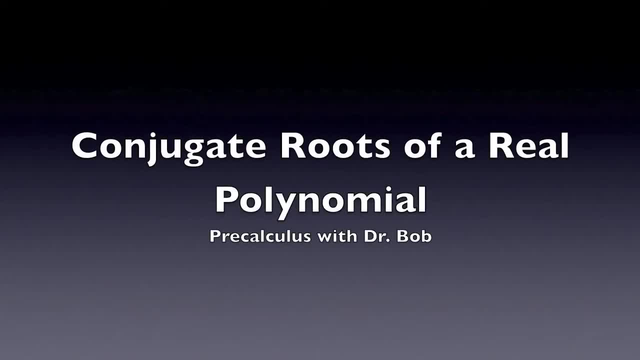 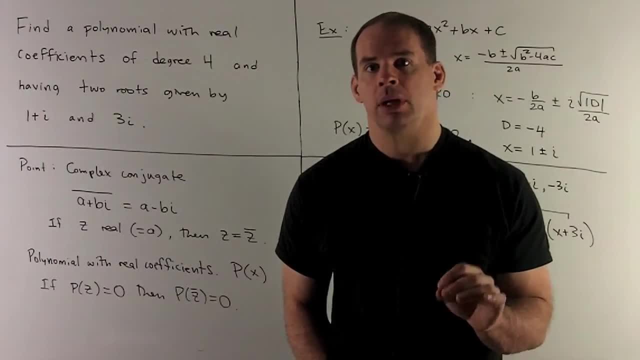 Find a polynomial with the real coefficients of degree 4, which has as complex roots 1 plus i and 3i. The tool we're going to need is complex conjugation. So we have a complex number, z equal to a plus bi. where a and b are real, This complex conjugate is going. 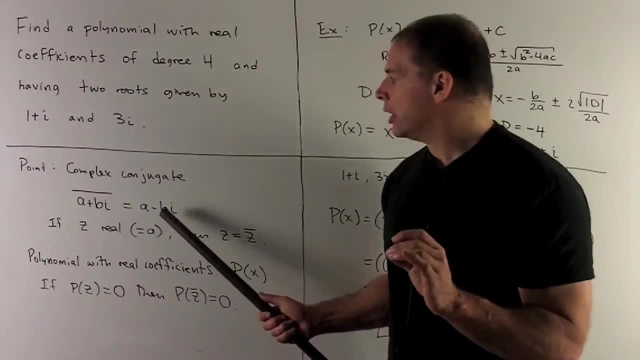 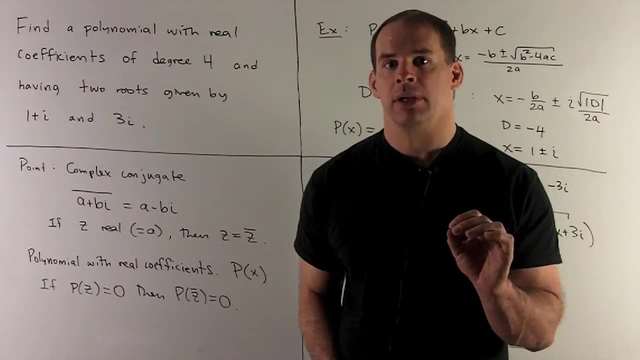 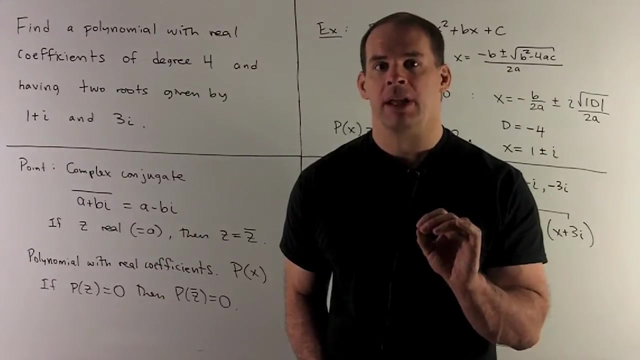 to be given by a minus bi. So all we're doing is taking the imaginary part, the part that has the i, and changing the sign. Now, if z is a real number, meaning it just has an, a, okay, just the real part- then its complex conjugate is equal to itself. So z equals: 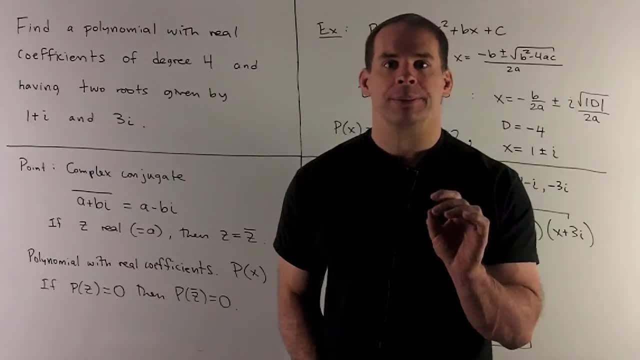 z bar. Next, if I have a polynomial with real coefficients, if I have a complex root, say a plus bi, then its complex conjugate is also going to be a root of the polynomial. So if a root is real, you take its complex conjugate, we do. 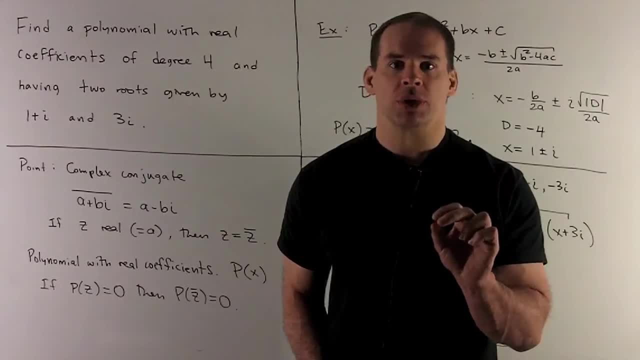 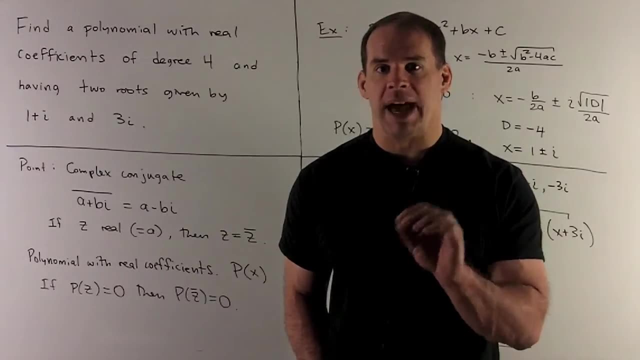 nothing, We just get the same root back. So for real roots, this doesn't really give us any idea of how to get new ones. But if I have a complex root, a plus bi, where b is non-zero, so we have a non-zero imaginary part. 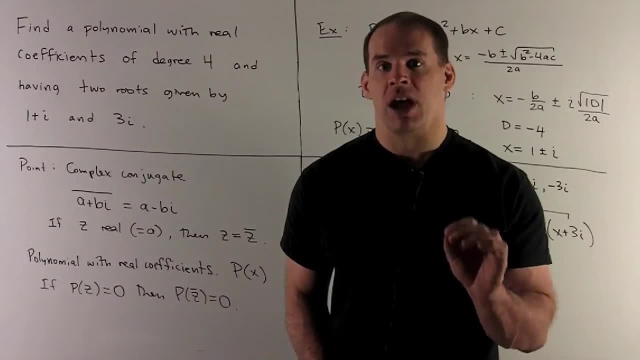 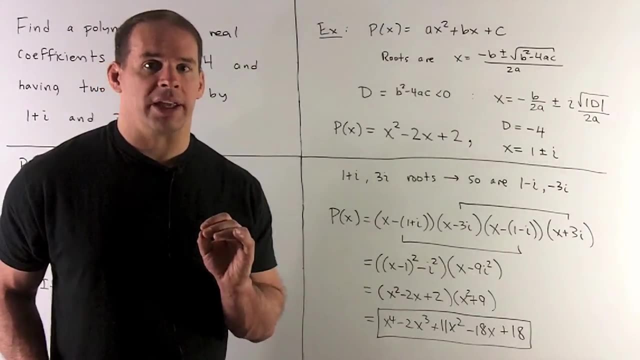 Then complex conjugation is going to give us another root of our polynomial. That's what we're going to need here. A good way to see this: use the quadratic case. So I have ax squared plus bx plus c. I want its roots, So we use the quadratic equation. 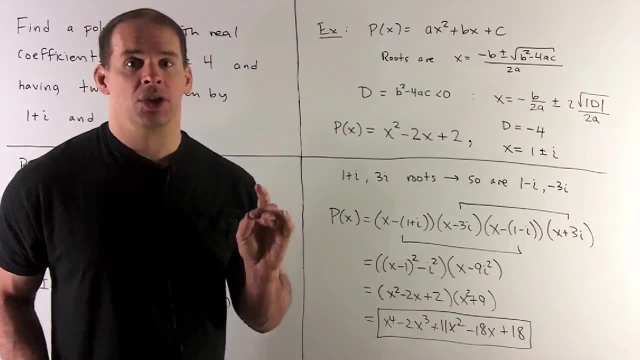 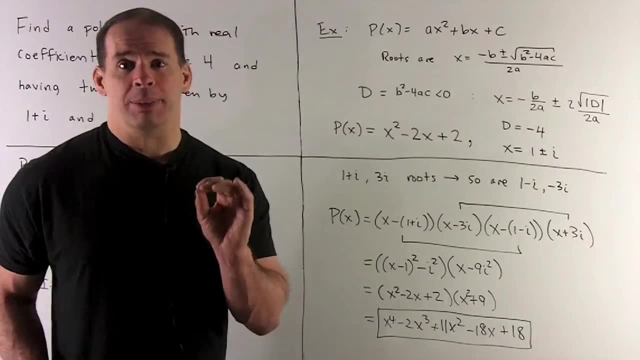 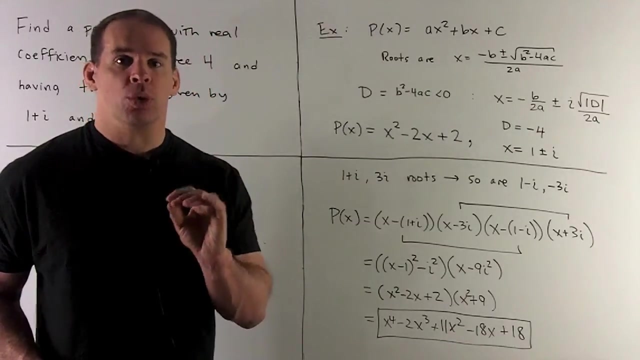 That gives me x equal to minus b plus minus square root of b squared minus 4ac all over 2a. This gets interesting when I'm looking at the root: b squared minus 4ac is negative. So in that case let's call it d. Then the roots: 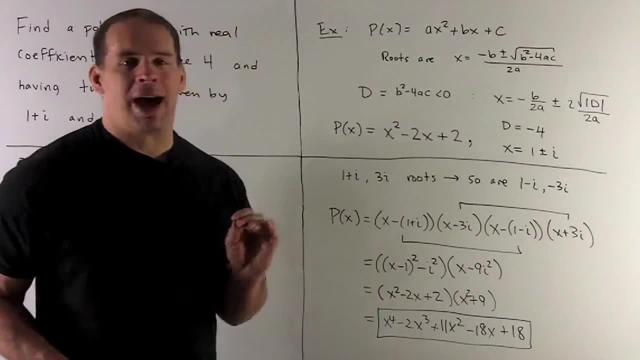 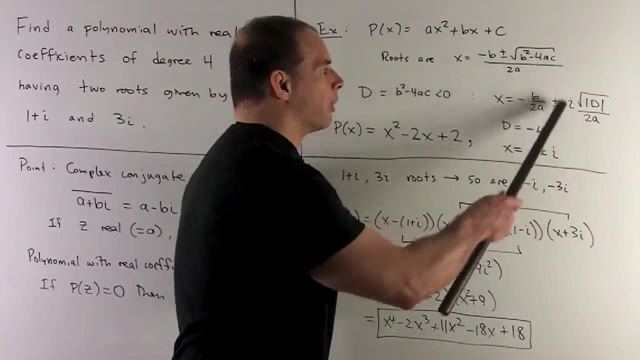 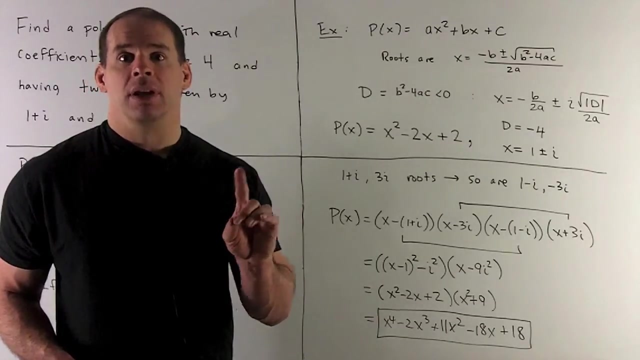 will be minus b over 2a. plus minus i times square root of the absolute value of d over 2a. Now this is just being proper about things. d is negative. I want to get the minus sign out of there. Square root of minus 1 is going to be i. That's how we define i And just. 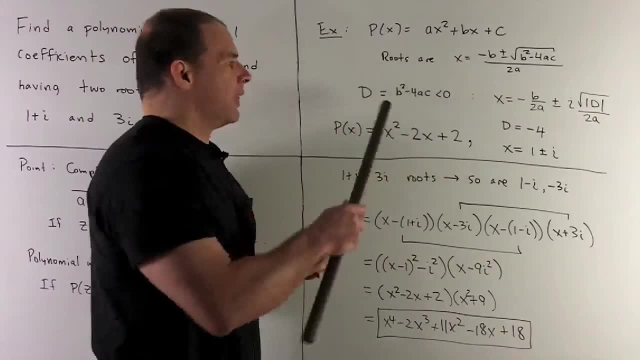 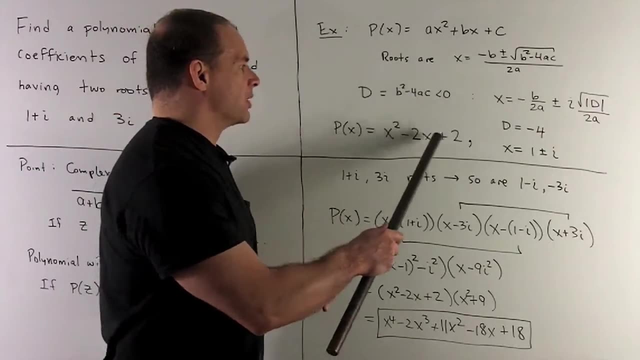 note: absolute value of d is just negative, This number without its minus sign. So think of the concrete example. If I take x squared minus 2x plus 2, what do we have? Your d is going to be minus 4.. So we're just going. 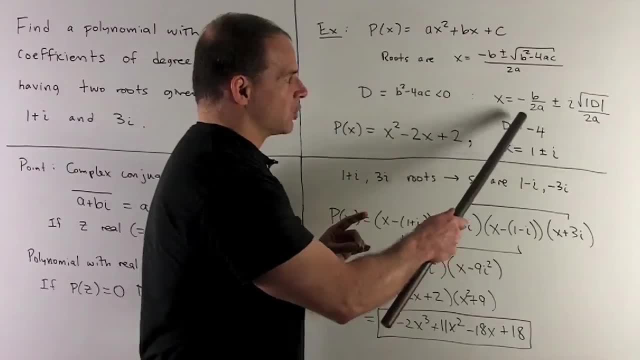 to pull out That's going to have. I'm going to take the square root. Square root of minus 1 gives me an i. Square root of 4 gives me a 2.. Then when I divide by 2a, that's going. 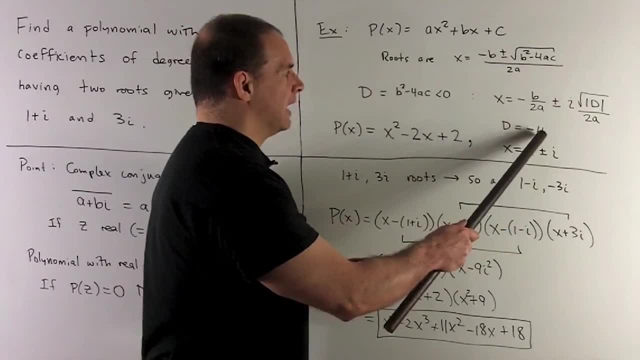 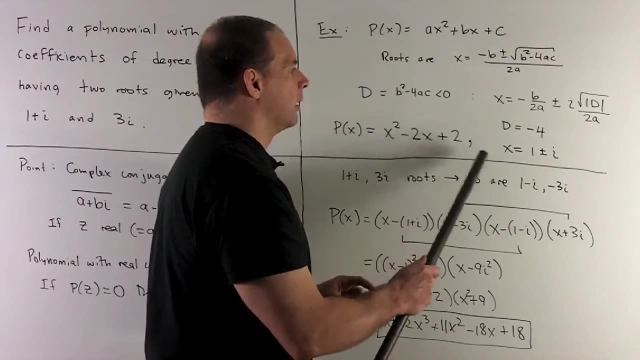 to be a is 1 here. Divide by 2 just gives me an i And then I have plus minus, Then I have a 1 for this piece. So that's going to be the roots of this guy, But you'll notice. 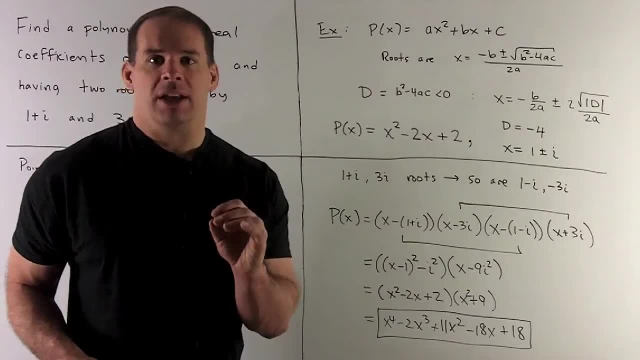 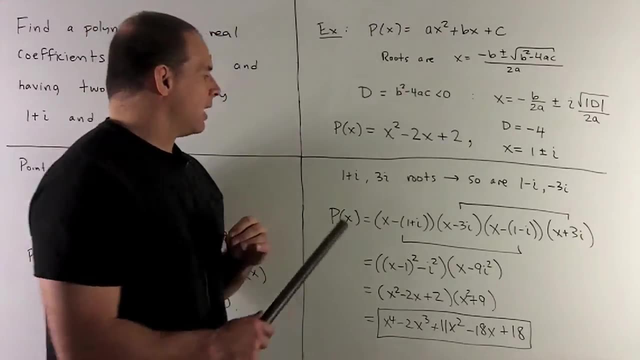 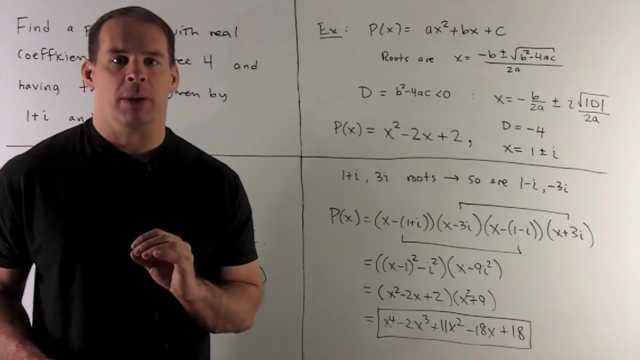 what's coming out is a pair of complex conjugate, complex numbers. Okay, So back to the original problem. I have 1 plus i, 3i as roots, So I have to throw in the complex conjugates if we want to have a real polynomial. So we'll have. 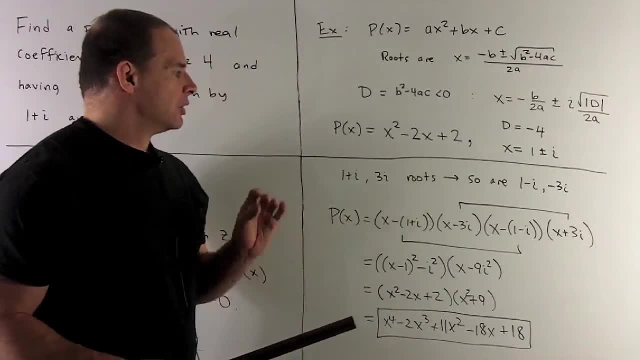 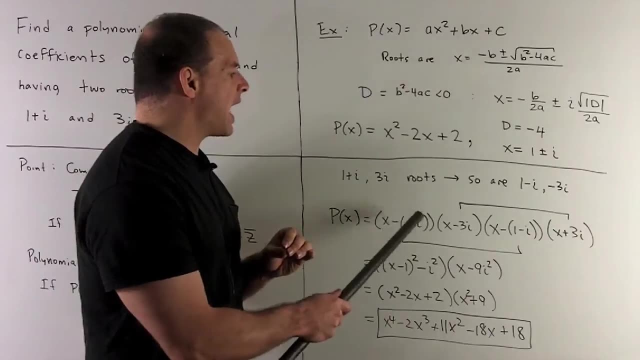 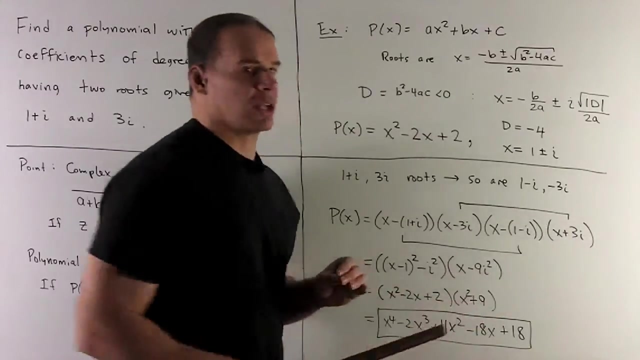 1 minus i and minus 3i. So we're going to have four factors, Four factors coming from them, roots. So it's going to be x minus your root. So I have x minus 1 plus i, x minus 3i, x minus 1 minus i, Then x minus a minus 3i, which is x plus. 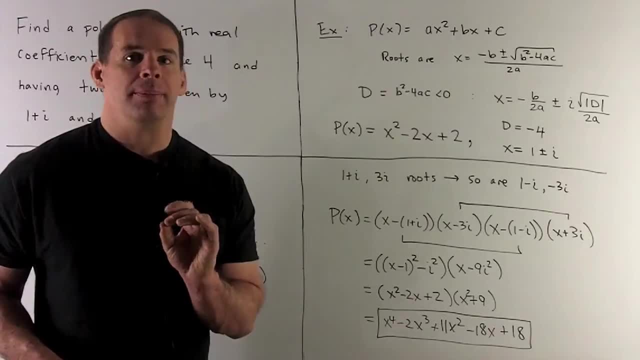 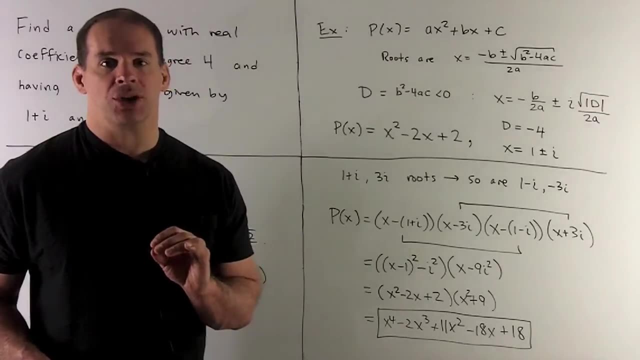 3i, The easiest way to multiply this out. okay, you can grind it out, But it's better to pair the conjugates together, So that way you're going to have differences of two squares. So, for instance, if I take x minus 3i, x plus 3i gives me x squared minus 3. 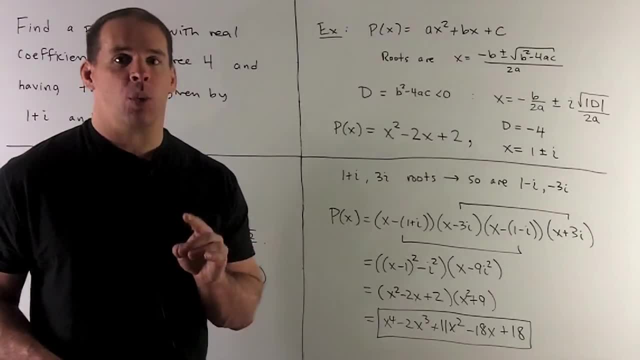 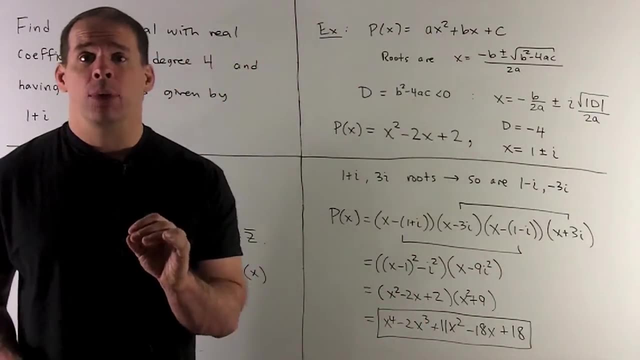 squared. I squared is minus 1.. So that becomes x squared plus 9.. For the other pair, you can grind that out Or you can notice I can write these as x minus 1 plus minus i, Then your. 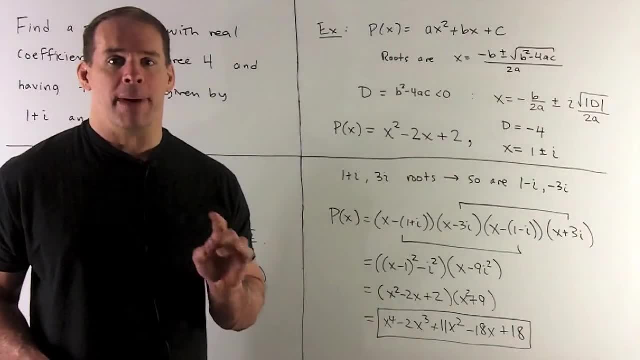 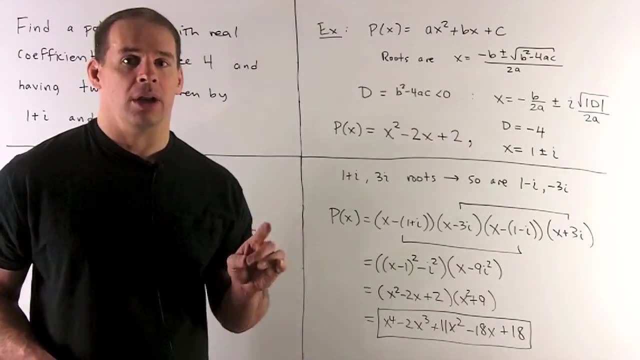 difference of two squares is going to be x minus 1, squared minus i squared. Okay, i squared is minus 1.. So this is x minus 1, squared plus 1.. Or x squared minus 2x, So this is: